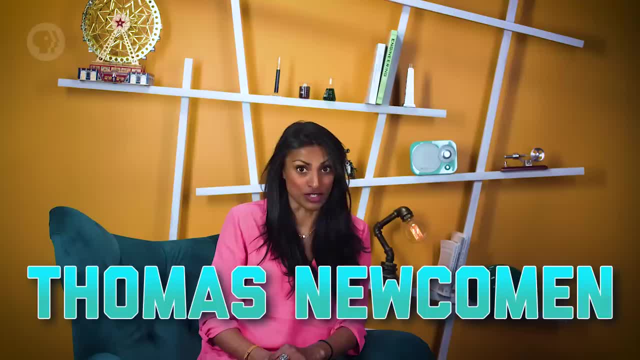 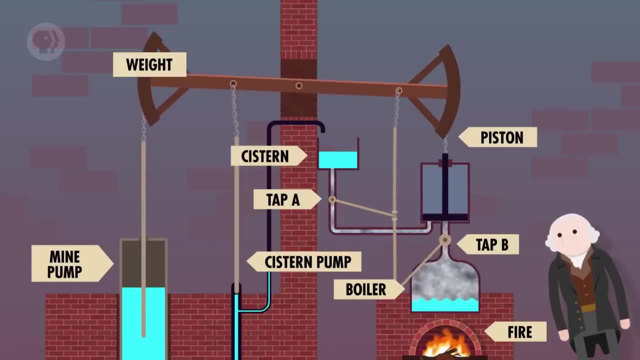 This brings us to Thomas Newcomen, a British inventor, who developed the first successful steam engine with a piston in 1712.. In his design, atmospheric pressure pushed the piston down after the condensation of steam had created a vacuum in the cylinder. 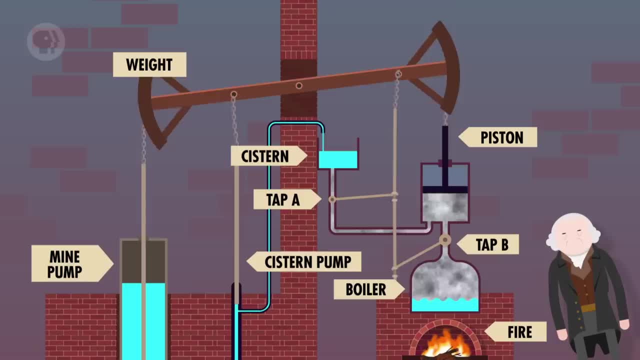 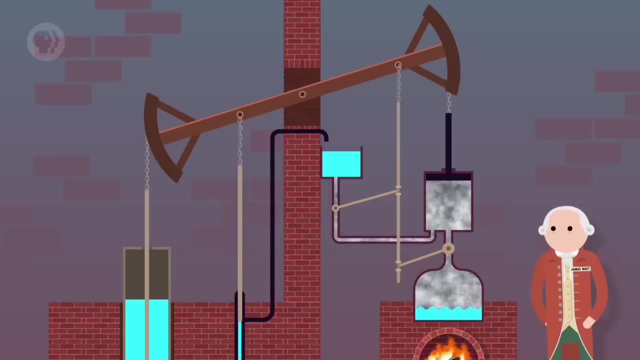 Its original use was to draw water out of the piston. This was part of the Cornish tin mines. after Newcomen found how expensive it was to use horses to pump the water, Then along came the Scottish inventor James Watt. In 1763, while repairing one of Newcomen's engines, Watt realized that about three-quarters of the energy from the steam was going to waste, used only to heat the chamber of the engine. 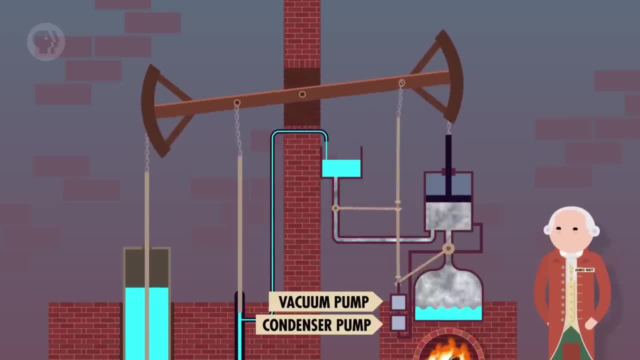 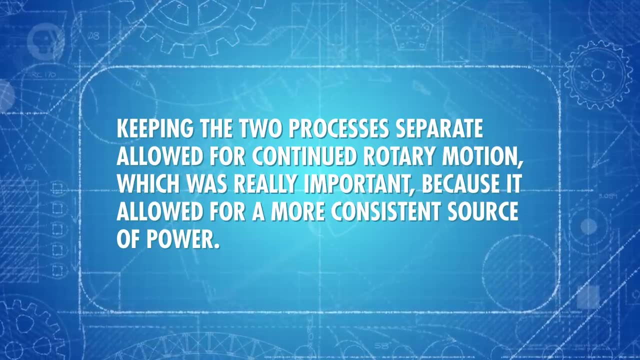 His solution was to have a separate condenser. The steam would then be condensed in a chamber separate from the piston chamber so that the condensed steam didn't go to waste. Keeping the two processes separate allowed for continuous heat. This allowed for continued rotary motion, which was really important because it allowed for a more consistent source of power. 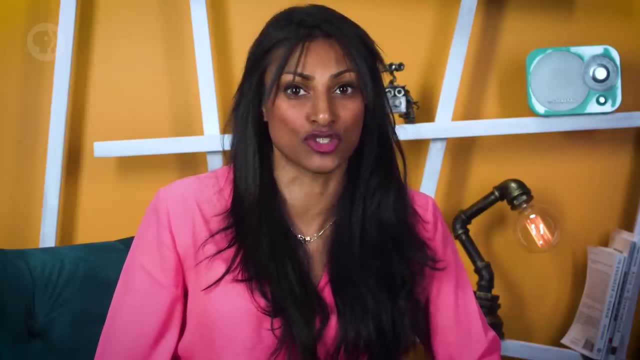 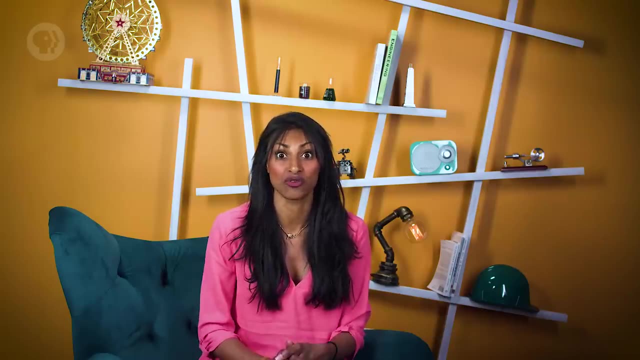 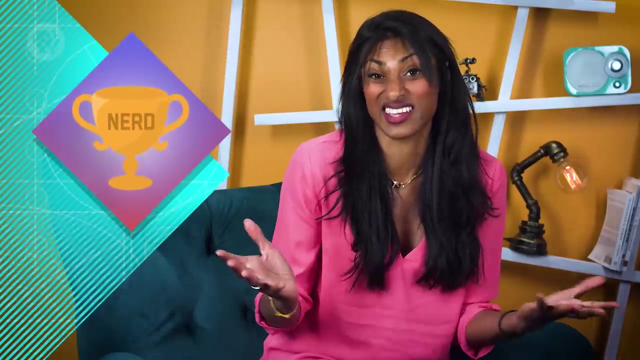 Watt's invention came to be widely used to run machines in the factories that drove the Industrial Revolution. Watt went on to be the first engineer to be commemorated in Westminster Abbey, with a large white marble statue erected in his memory. He also had his last name recognized as a unit of power, which is perhaps one of the highest honors that an engineer can get. But steam engines really came into their own, especially in the realm of transportation, in the locomotives of the 19th century. George and Robert Stevenson, an English father-son duo, are famous for their early steam locomotive, which they called, aptly enough, locomotion. 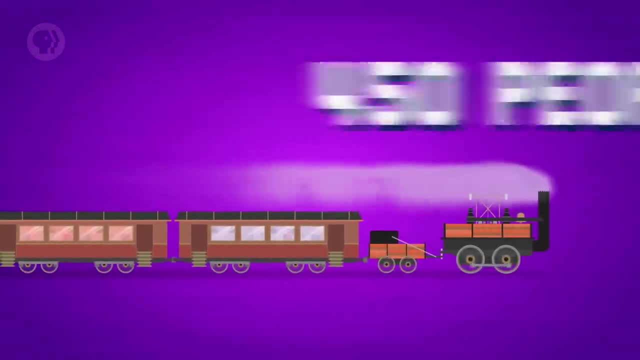 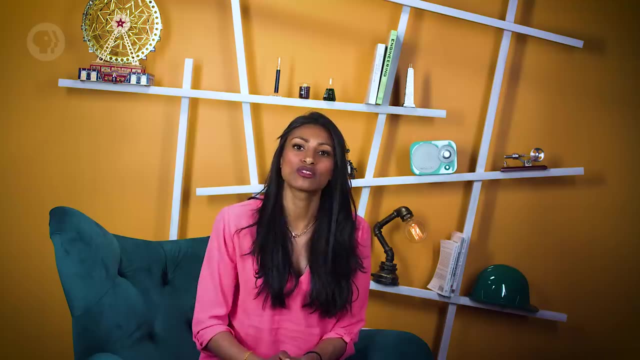 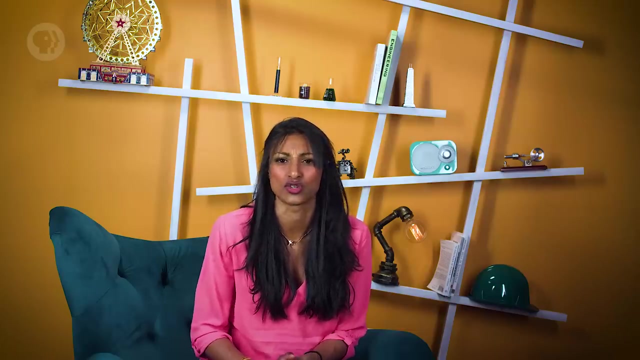 In 1825, it became the first public passenger train carrying 450 people at 24 kilometers an hour – quite a bit faster than a horse. But while wheeled vehicles allowed people to travel more quickly, on land, transportation was still limited by bodies of water and rough mountainous terrain. 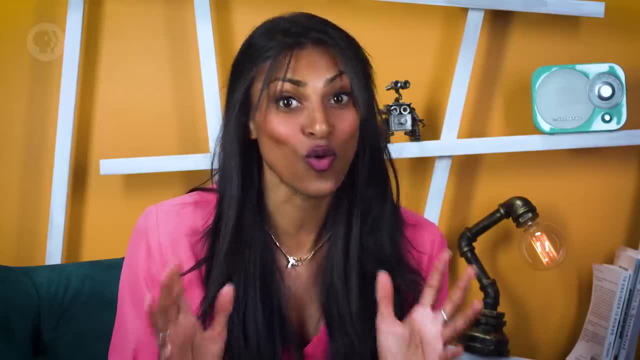 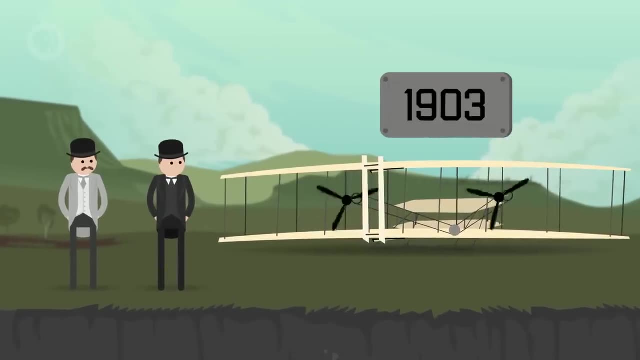 If engineers could figure out a way to get people to fly, all of that could be avoided. This problem-solving led to the invention of aircraft. The first powered aircraft to take flight was the Wright Flyer in 1903, which was designed by Wilbur and Orville Wright and used a 12-horsepower gas engine. 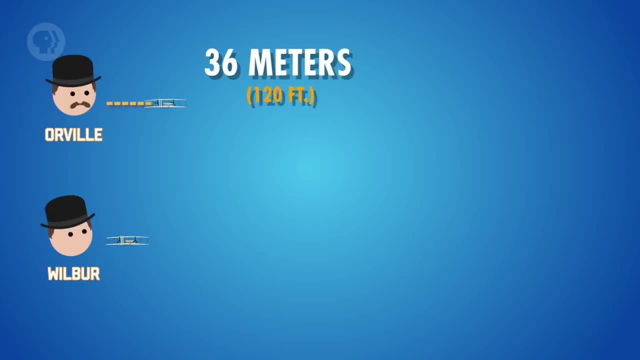 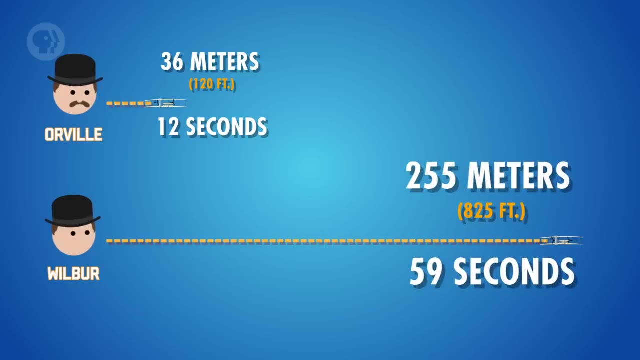 Orville flew the Wright Flyer on its maiden voyage, traveling 36 meters in 12 seconds. but the best flight of the day belonged to Wilbur, who traveled over 255 meters in 59 seconds, or a speed of about 15 kilometers an hour. Earning him some serious bragging rights. Soon after the Wright brothers' accomplishment, World War I sparked a burst of aircraft innovation. Engineers began using metal in structures of airplanes and better engines, allowing them to reach higher speeds and altitudes. Then, in 1930, Sir Frank Whittle obtained his first patent for a turbojet engine. But it wasn't until the outbreak of World War II that the British government had a compelling reason to support his work. By 1941,, Whittle's engine featured a multistage compressor, a combustion chamber, a single turbine and a nozzle, which was a big improvement, since previous engine designs only had an internal combustion engine and a propeller. Jet engines outperformed the older designs, flying farther, faster and cheaper too. These advances ultimately made commercial air travel possible, and soon. people were traveling where once only the birds had ruled. But mechanical engineering doesn't stop in the air. 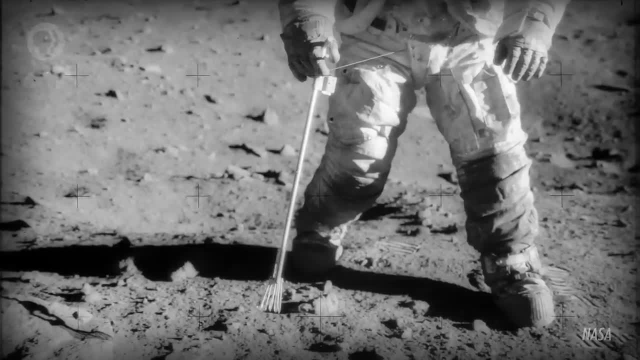 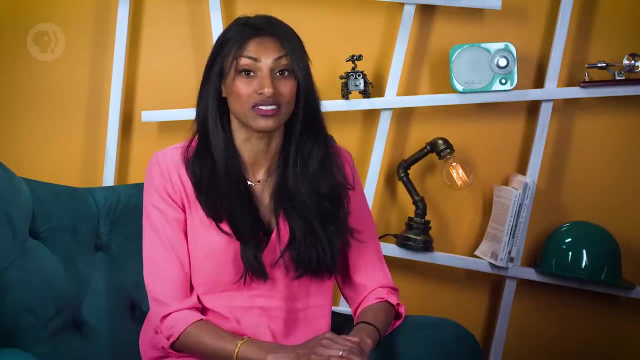 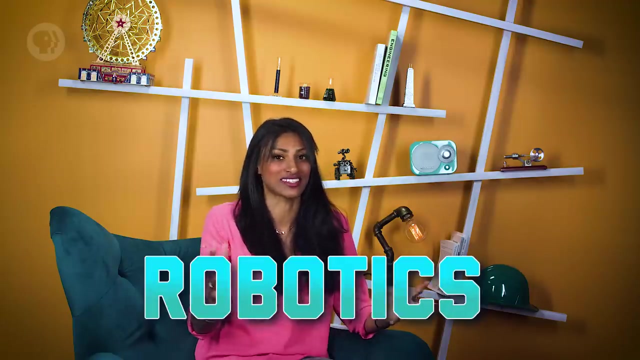 Beyond planes, we've sent satellites into orbit, astronauts to the Moon and spacecraft carrying rovers all the way to Mars. The aerospace side of engineering actually arose from the mechanical field, And much of what has allowed us to build these machines that move us is another big part of the mechanical engineering field – robotics. 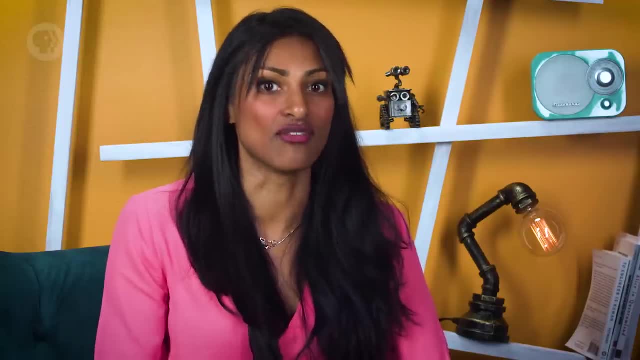 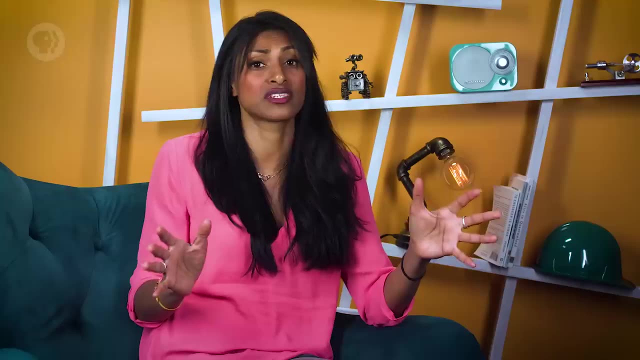 For most of industrial history, humans have been at the center of our workforce. But humans have their limits. Some things are too big and too awkward to move, while other processes need finer precision than the human hand allows. Industrial environments are also often uncomfortable and sometimes even dangerous. 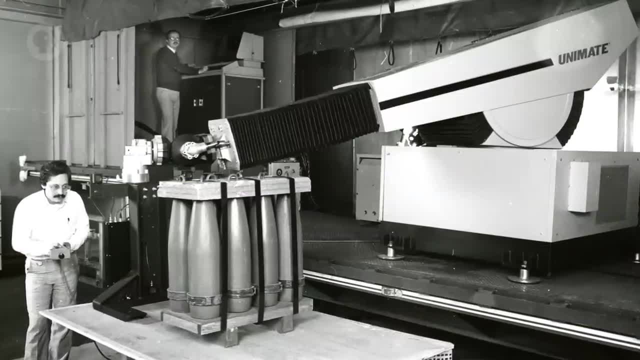 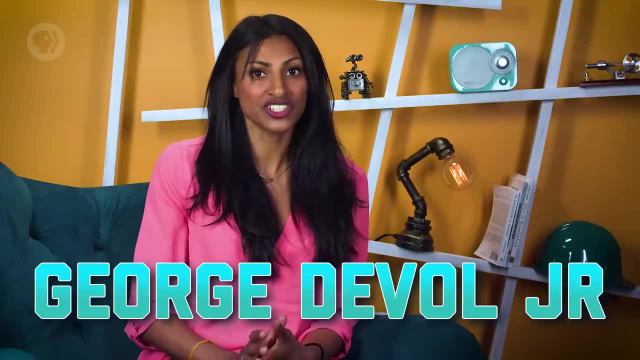 And that's where robots and automation come in. The first industrial revolution was in the 1930s. The first industrial robot, called Unimate, appeared around 1960. It was designed by American inventor George Duvall Jr, who worked with engineer and entrepreneur Joseph Engelberger to get it into factories. 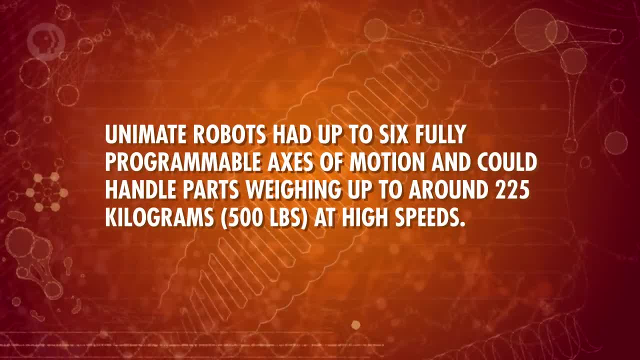 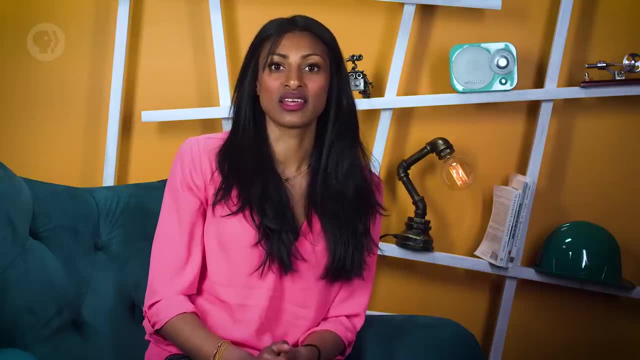 Unimate robots had up to six fully programmable axes of motion and could handle parts weighing up to around 225 kilograms at high speeds. They soon joined the assembly line at a General Motors plant, where they took die castings from machines and welded them onto autobodies. 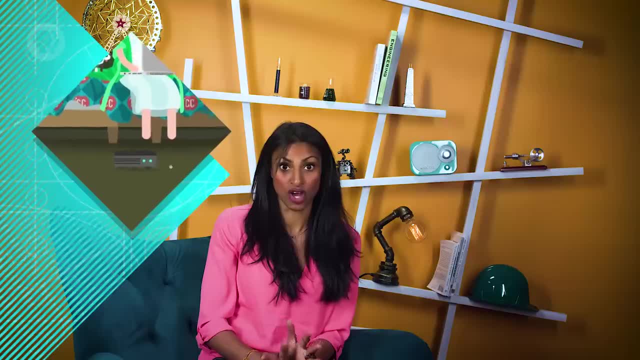 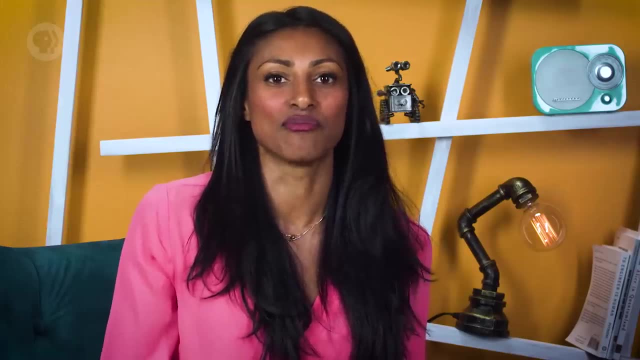 Since then, robots have gone beyond space- Some of their 쓰는 elements are- As well. they're used in road manufacturing, showing up in our homes to clean the floors, and even hospitals to perform surgeries. But as their applications get more advanced, engineers have more and more factors to consider. 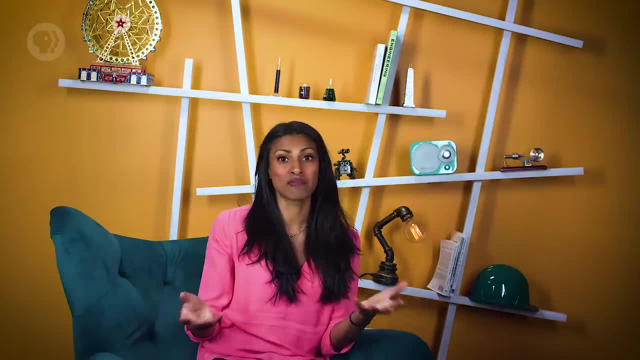 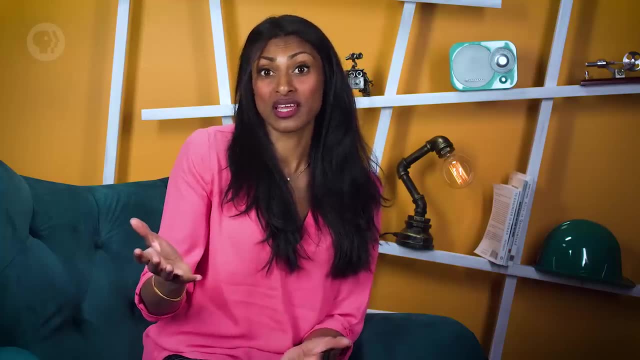 They need to worry about how well robots sense their surroundings, how they move and manipulate their environments, and much more. It's possible one day that you'll have robots in many of the places you could imagine a human working. I mean, we're seeing that now. 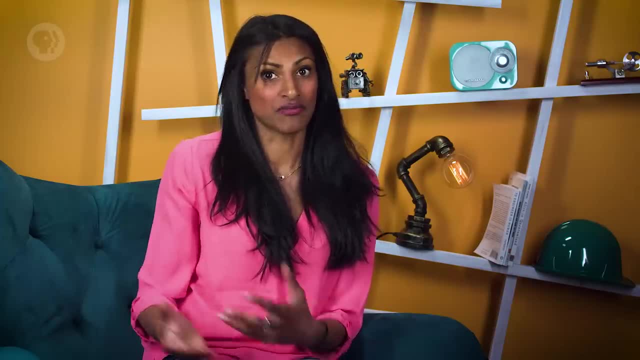 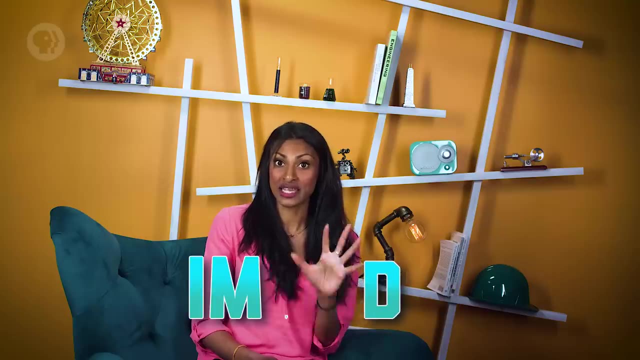 And speaking of humans, you can think of the human body as just a super-complex mechanical system of its own connecting joints, and this is where biomechanics comes in. Engineers need to take into account the stress, load and impact that our bodies can withstand. 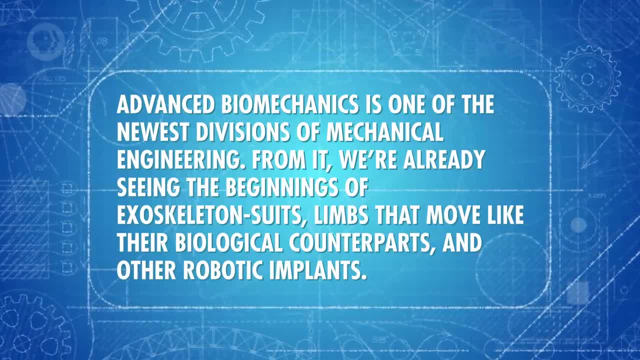 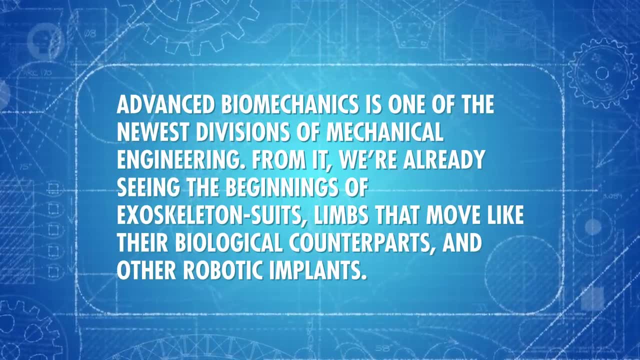 and apply it to machines that are modeled on us. Advanced biomechanics is one of the newest divisions of mechanical engineering. From it we're already seeing the beginnings of exoskeleton suits, limbs that move like their biological counterparts, and other robotic implants. One of the more impressive projects is the Berkeley Lower Extremity Exoskeleton, Founded by the Defense Advanced Research Project Agency in 2000,. this device is designed to provide mechanical support to allow nearly anyone to carry larger, heavier loads than they could ever lift on their own.